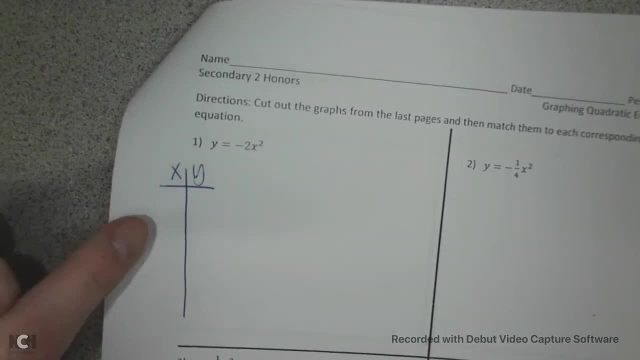 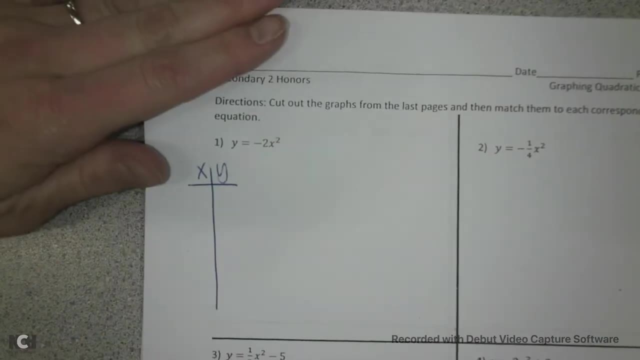 So there are other methods. One of the easiest methods is to create a table of values. Okay, and then I'm going to show you a few different types of methods that you could use to figure out what graph belongs with which equation. So I'm going to pick some numbers. 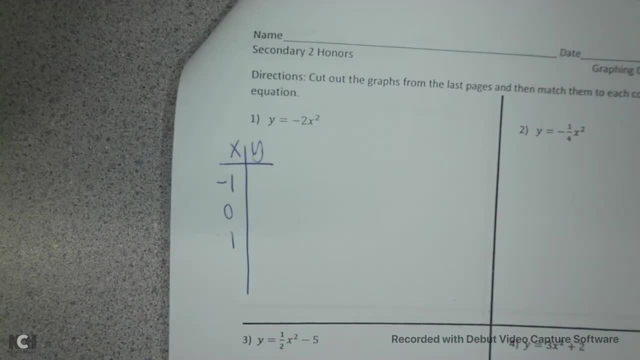 really fast. I'm going to pick negative 1,, 0, and 1.. I'm going to start with those and kind of see what we get, and then maybe we'll have to adjust. We're just going to see. So if we plug in negative, 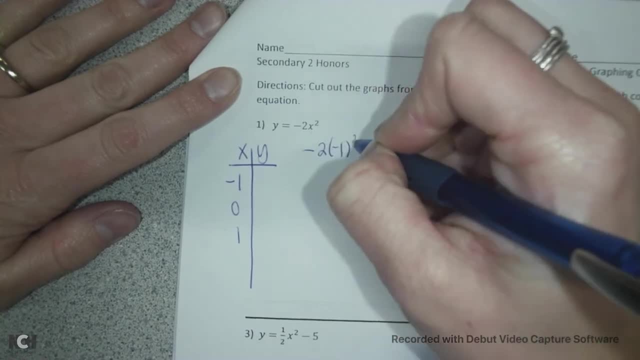 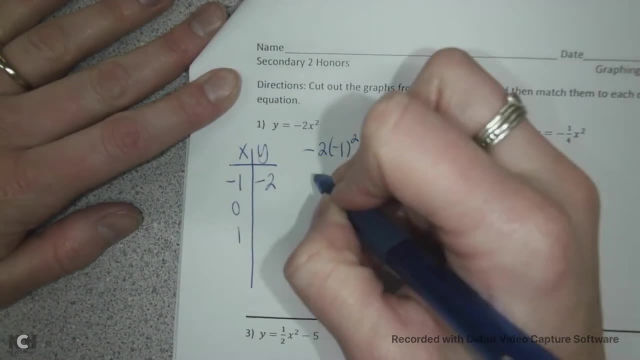 1 to where our x is. so we have negative 2 times negative 1 squared. Negative 1 squared is 1.. 1 times negative, 2 is negative 2.. Then, if I plug in 0, negative 2 times. 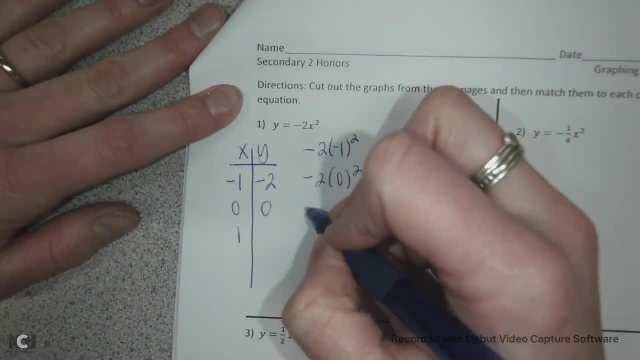 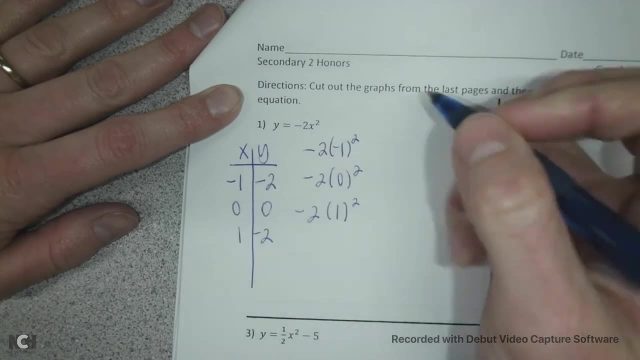 0 squared, well, that's going to be 0.. And then if I plug in positive 1,, so 1 squared is 1 times 2, negative 2.. Okay, so I have some nice ordered pairs that will probably fit on my graph. 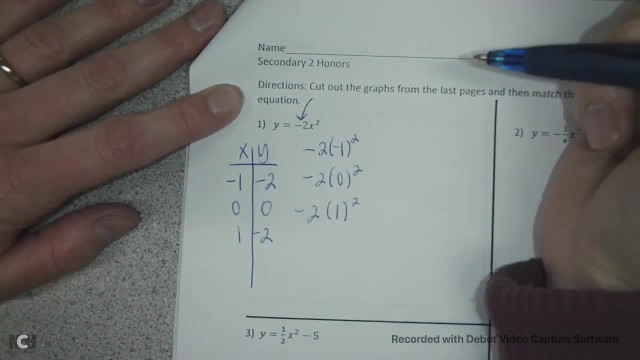 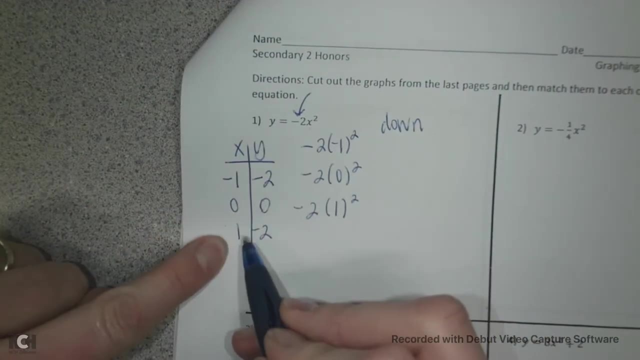 Then we're going to look at our a value, So the number in front of your x squared. if it's negative, remember- then our graph is going to open up down. So I should have a dot at 0,, 0, and then let's just go with this one: 1, negative 2.. So our x value. 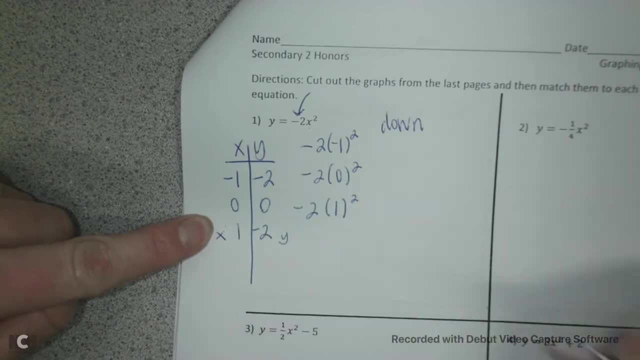 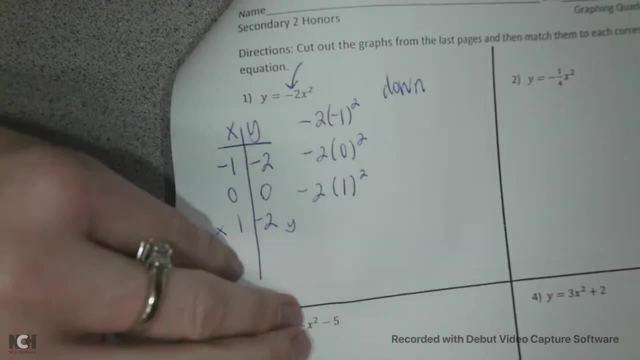 is 1,, so we go right 1, and then we're going to go down 2, because that's our y value. Okay, so 0,, 0 opens down, and then 1, negative 2.. So that's what we're looking for on our graphs. 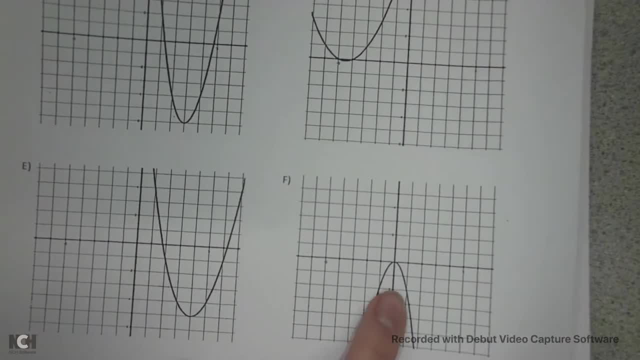 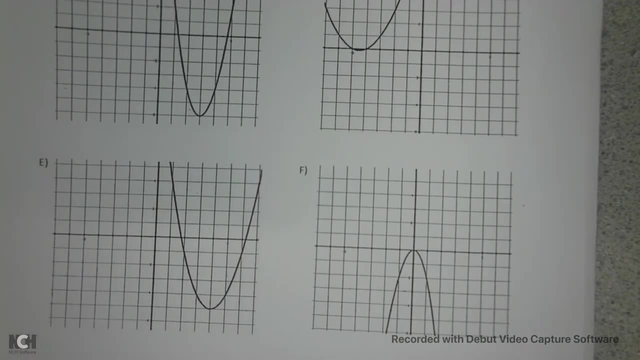 So 0, 0,. none of those. Oh, this one is 0, 0.. 1, negative 2 opens down, and then it's negative 1, 2.. Yep, this is it. So f belongs with number 1, and that is f. 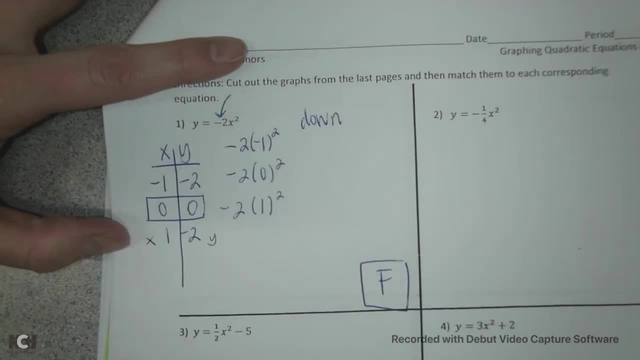 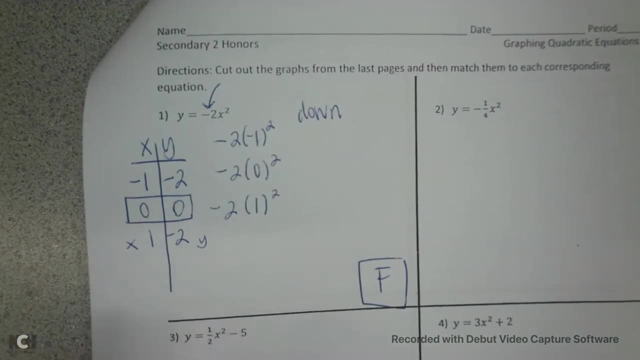 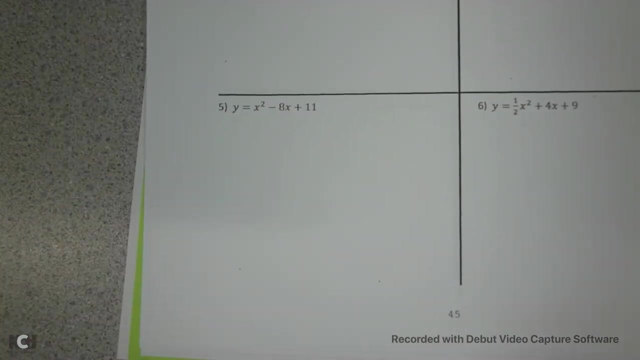 Okay, so this guy is our vertex. So then you would cut out that and glue that here, Or you can just write these by it. It's really not a big deal, It's just more fun to glue it. Okay, let's look at number 5.. So on number 5, we learned about writing the vertex. 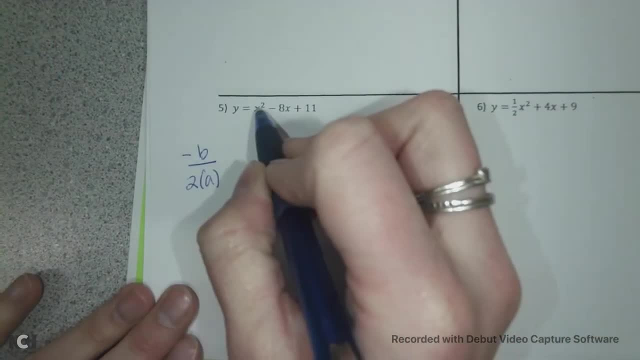 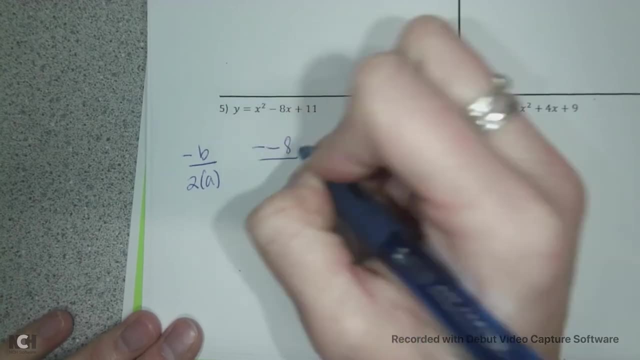 using negative b over 2a. Well, I have that information here and I'm going to use that here, So why not? Okay, so negative b is negative 8 over 2 times 1.. So negative 8, that's positive. 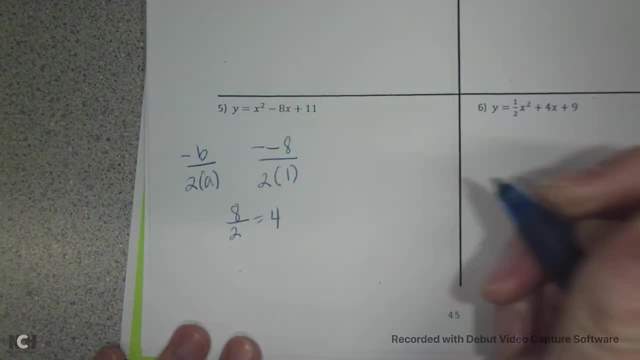 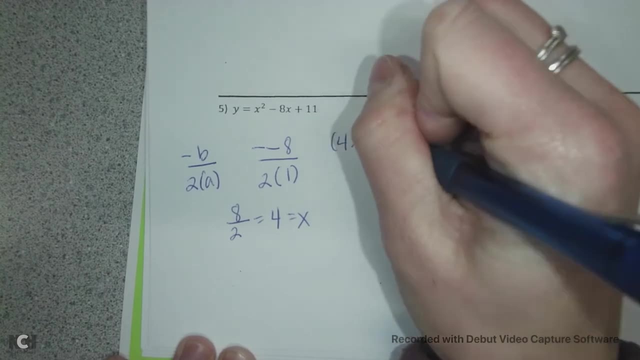 8 divided by 2 is 4.. Okay, so that is my x value and I'm going to plug that back in here. So I have 4 squared minus 8 times 4 plus 11, and I just don't want to think about it. 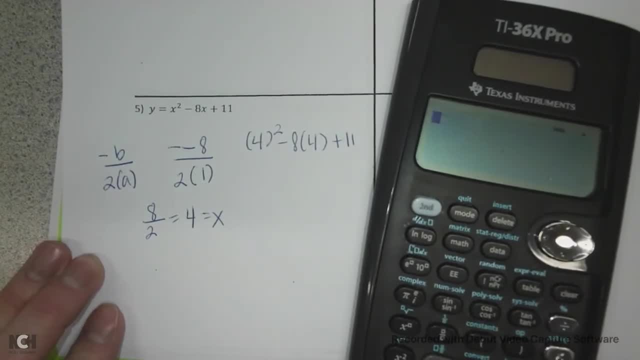 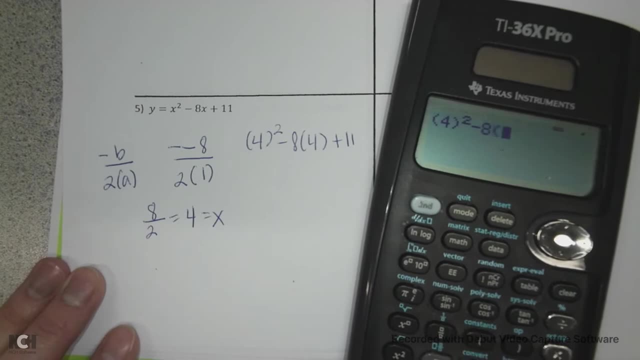 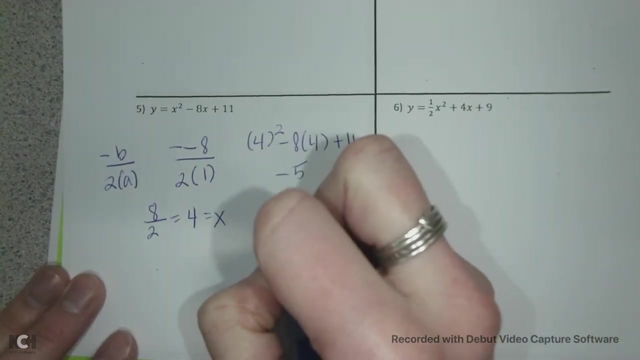 so we are going to use our calculator. So 4, just be careful when you square. if you square negatives, Two negatives multiplied together make a positive. Be very careful. Okay, so negative 5.. So my vertex is at 4,, negative 5, and since my a value is positive, 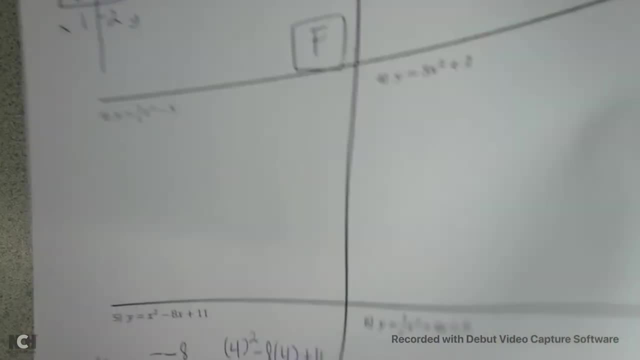 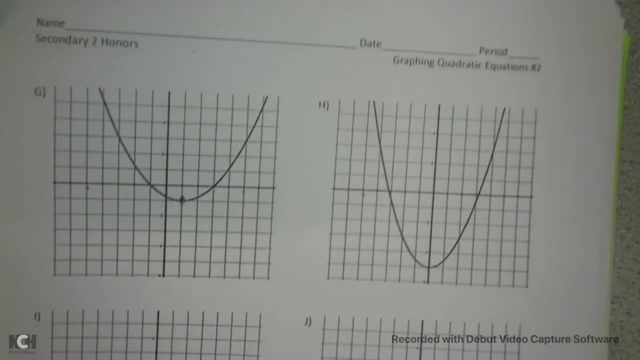 it opens up. So I'm looking for a 4, negative 5 that opens up Should be graph 5.. 4, negative, 5, nope, Alright, well, keep going. Oh heavens, I can't turn the page. Okay, 4, negative 5.. 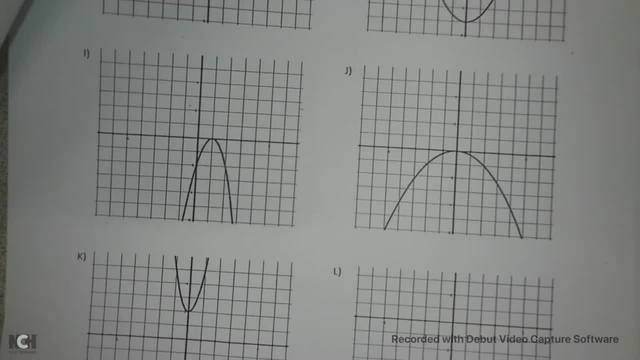 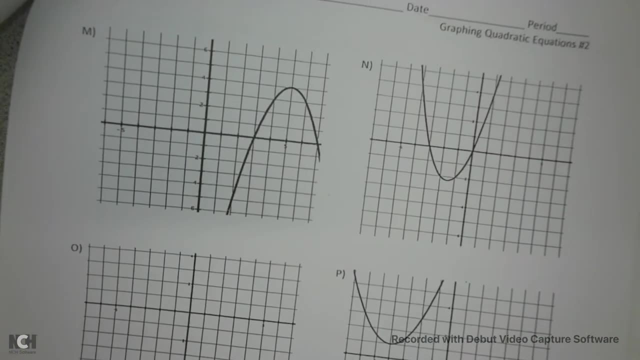 Oh-oh, did we do something wrong? To the right 4 and down five. hmm, To the right 4 and down 5, to the right 4 and down 5.. Oh, it just mixed. And here we go again. detected. 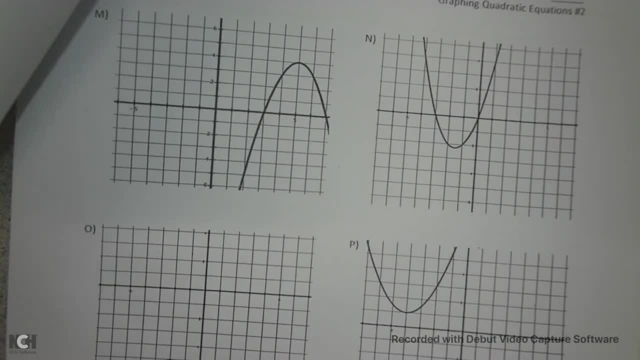 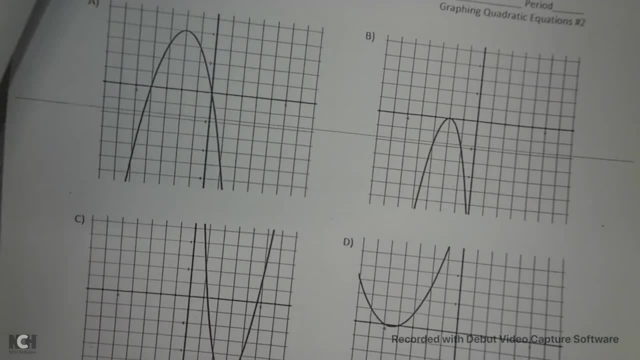 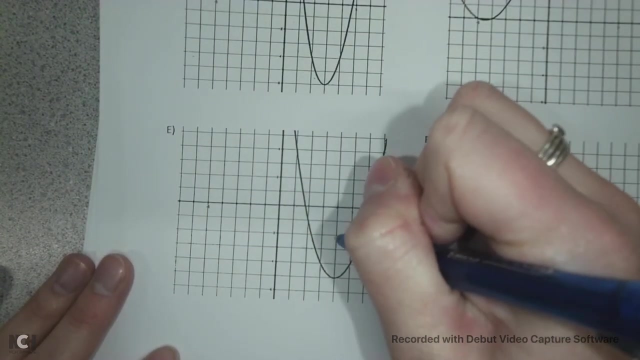 Decreased yet again. I have 4 squared and 5 negative, 5 times 1, 5 divided by 2, that's negative 9 plus 11.. Oops, Oops, Oops, Ouch, missed it. Okay, look at this guy. So, to the right, 1, 2, 3, 4, down, 1, 2, 3, 4, 5, it opens up. This is: 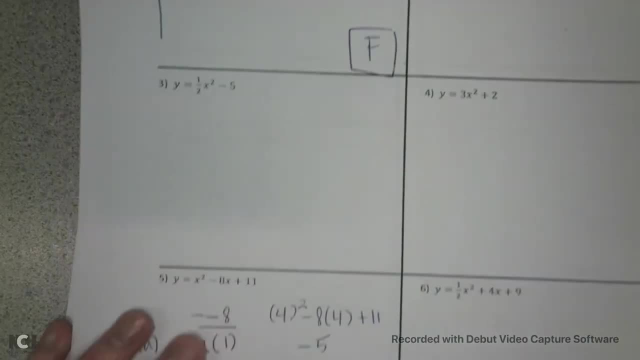 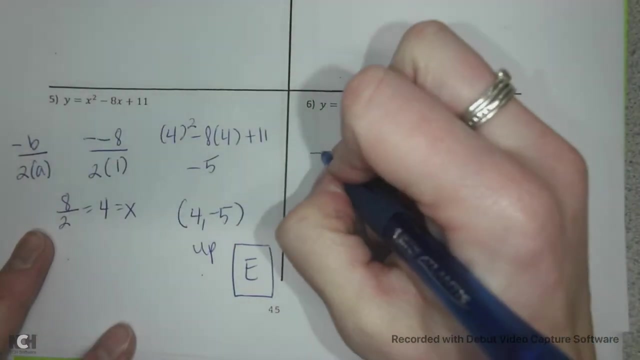 number 5.. It was e, I just went too fast, Silly Miss Nebby. Okay, so e matches 5.. So you could do the same thing on number 6.. You could do negative b over 2a to figure out the vertex, because again, 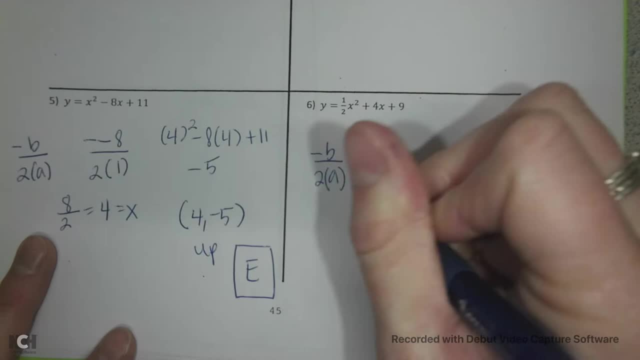 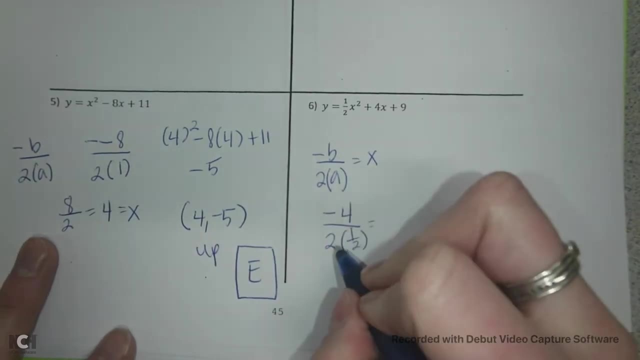 that's going to be the easiest and that's our x value. So negative b is negative 4 over 2 times 1 half. Well, negative 4, wait, 2 times 1 half half of 2 is 1, negative 4.. So negative 4 is our. 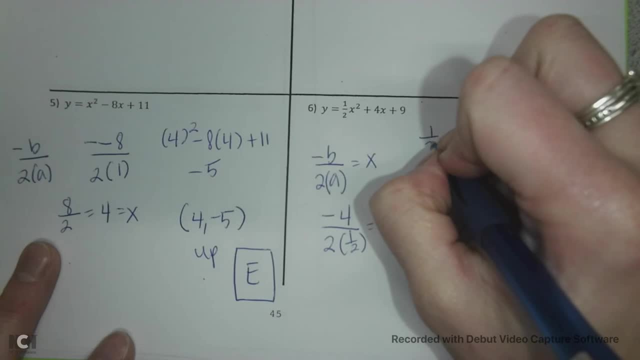 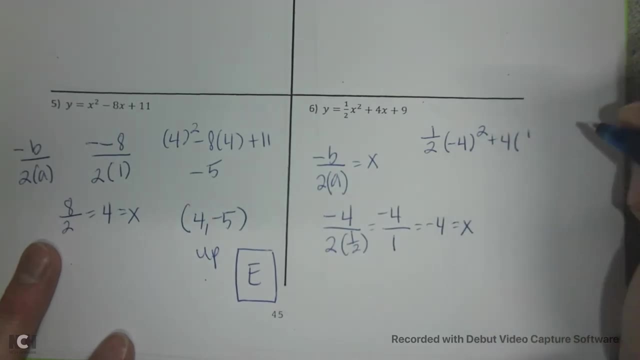 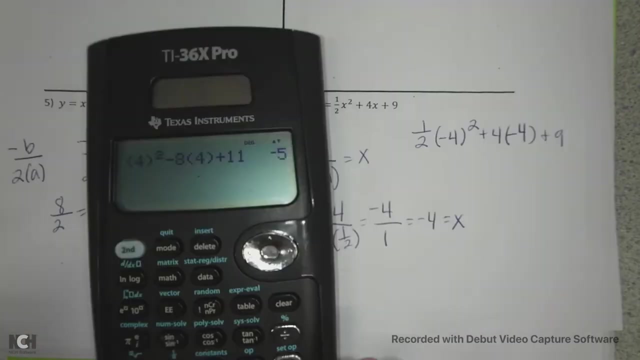 x value, So we're going to plug that in here. We have 1 half times. oh, definitely love that. I can show you this. Oops, x is our negative 4.. Yeah, look at me, Save that Plus 9.. Okay, now, when you type this in, please be very careful. Watch If I type. 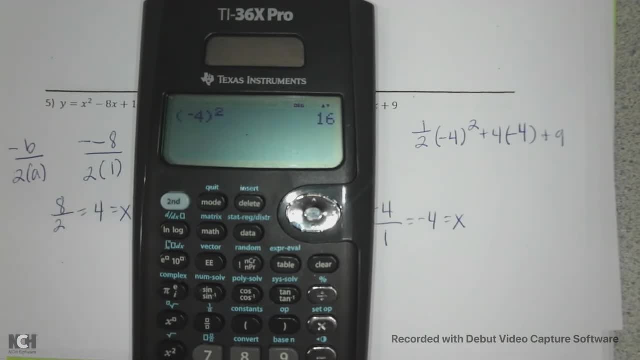 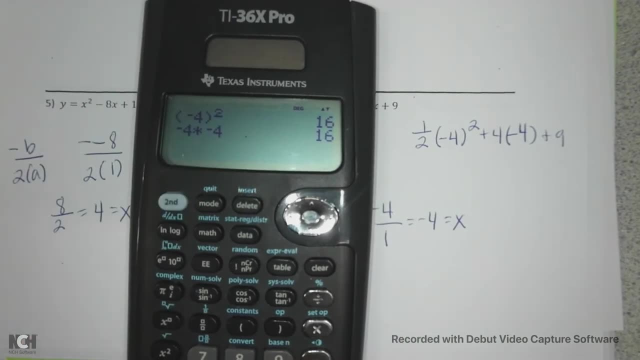 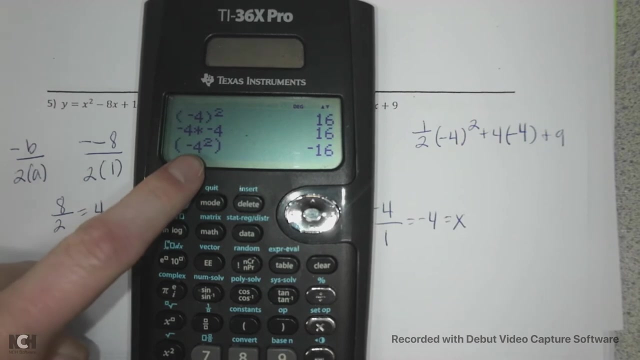 negative 4 in my parentheses and my square on the outside, I get the correct answer because negative 4 times negative 4 should give me a positive 16.. A lot of you forget and you do this: negative 4 squared, You're like, but why did it give me negative 16?? So right here, this guy in your 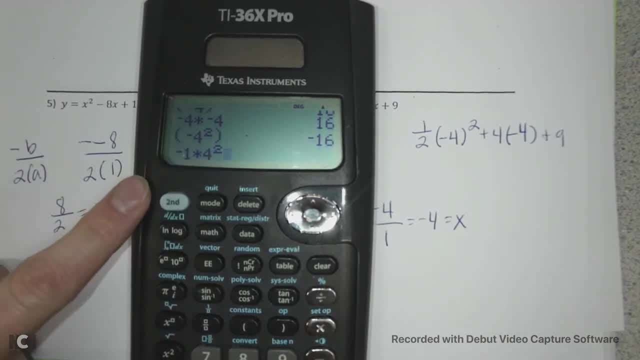 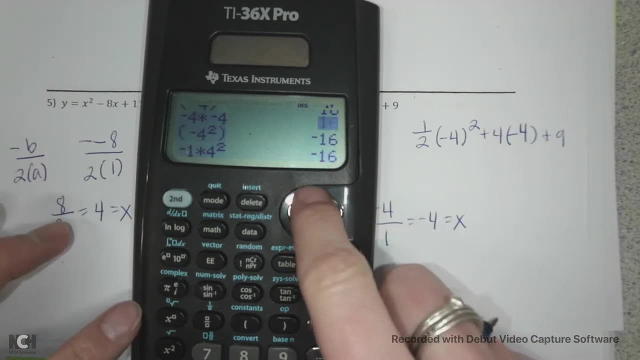 calculator. you're telling your calculator to do this. That's what you're telling your calculator to do, So that's why it gives you negative 16.. So parentheses are important. This is the best way where you have the negative 4 in parentheses and 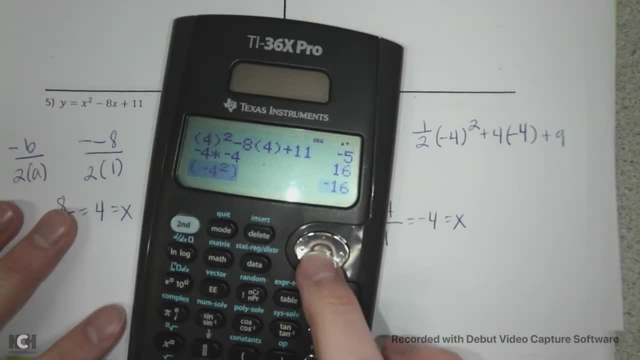 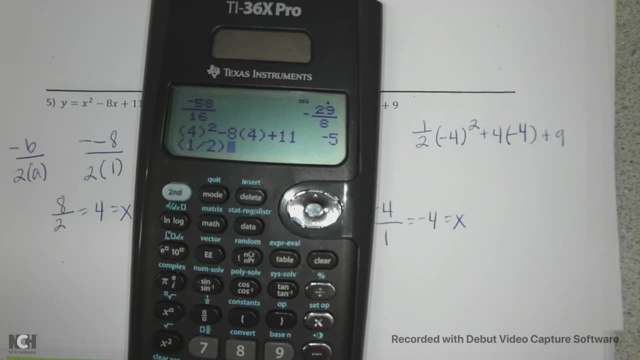 then squared on the outside, Okay so. oh yeah, that's right, I forgot what I was doing. I got so excited to show you. Okay, so I'm going to type 1 half. I like to put my fractions in my calculator. 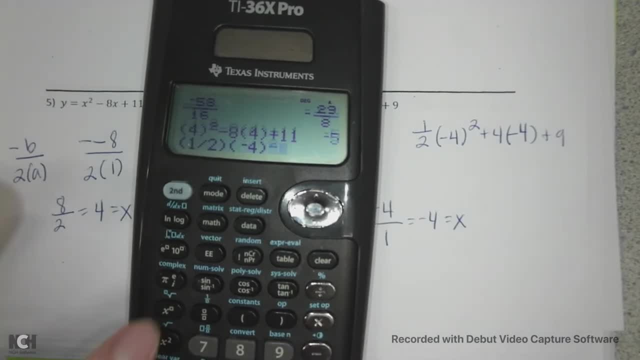 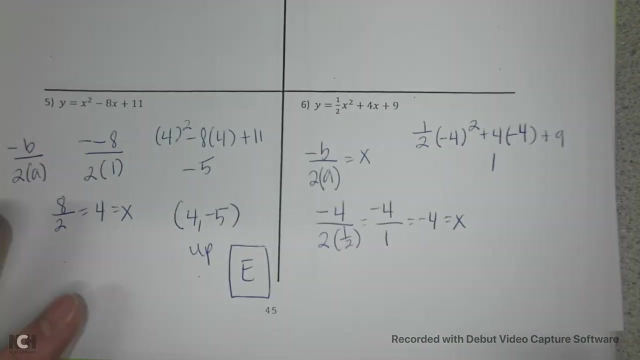 with parentheses. You don't have to, I just like to. I think it's because I learned on some old school calculators And that's what you had to do. So then, 4 squared plus 4 times negative, 4 plus 9, and I get 1.. Okay, so my 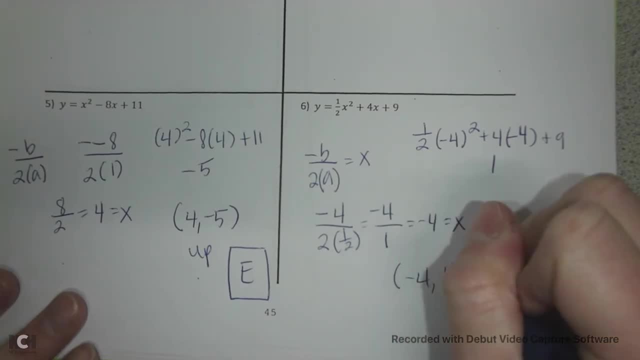 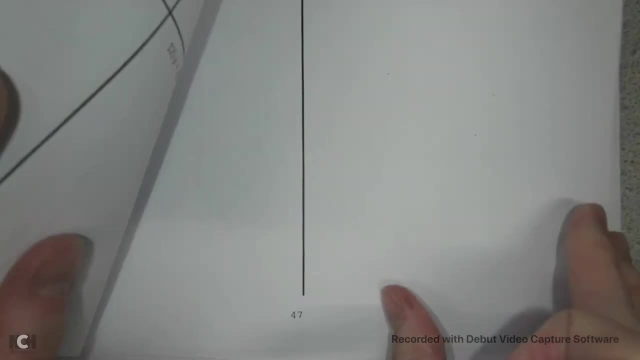 vertex for number 6 is going to be at negative 4, 1, because, remember, this is your y value And since my a is positive, it's going to open up. So, negative 4, 1, opening up, Good heavens. Negative 4, 1.. 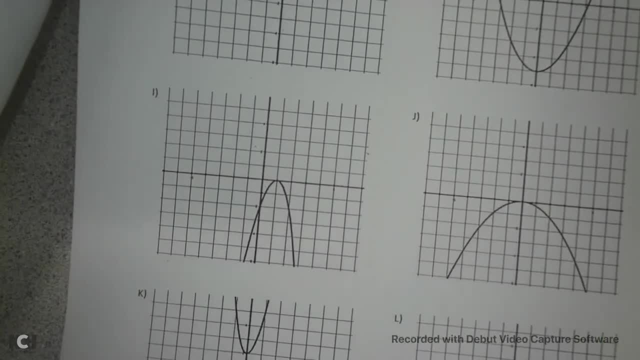 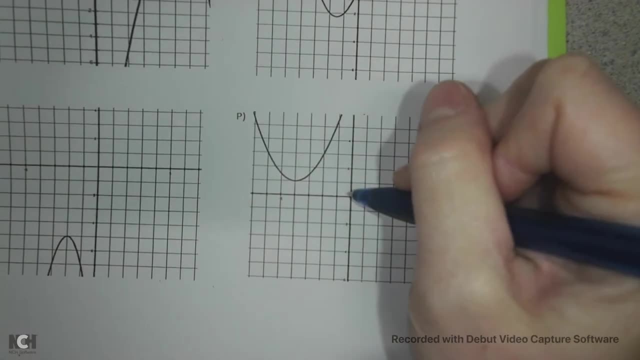 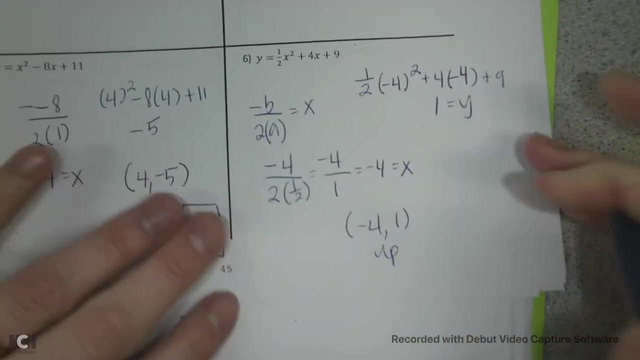 Those guys are not good. Negative 4, 1.. Not those guys. Oh there it is. Negative 4, 1. It opens up So that matches. So p matches with number 6.. So number 6 is p. At the very end you're going to have to take a quiz and tell me. 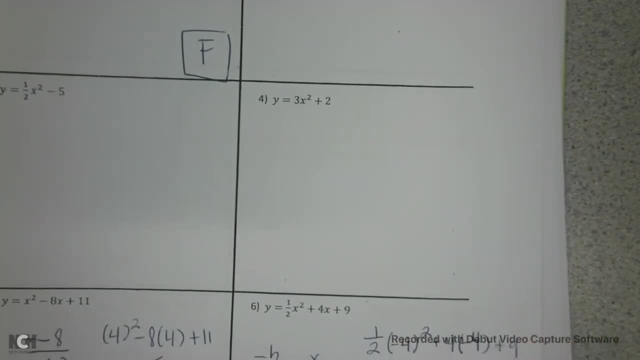 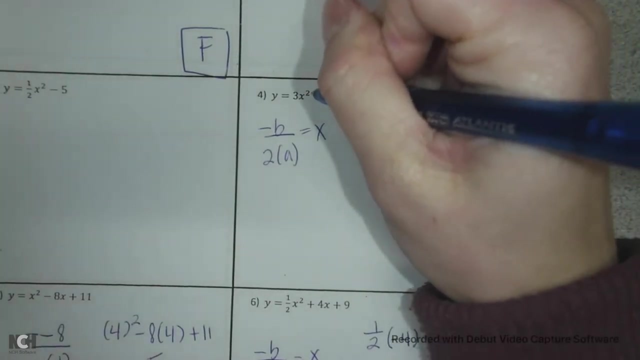 which ones match. Okay, if you wanted to try number 4 and do that exact same thing- or you do negative b over 2a- you totally could, Because that's our x value. Here's the thing When you don't have a middle term. so this is: 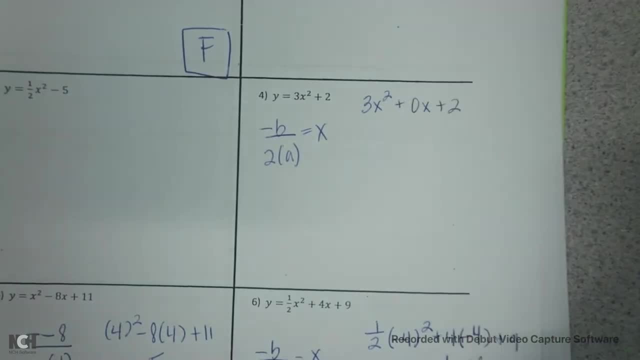 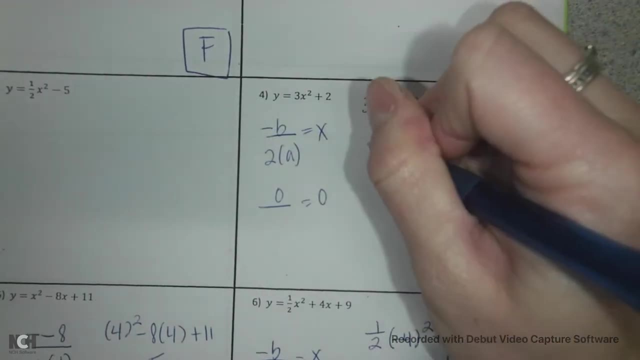 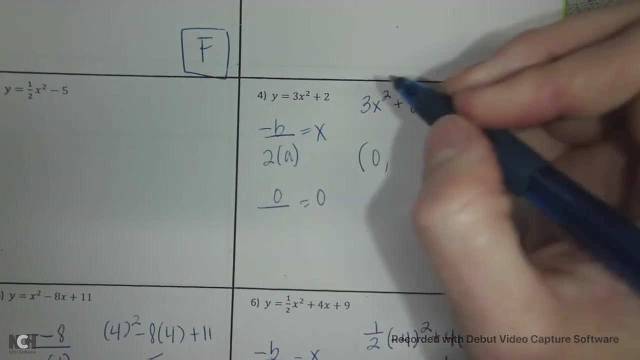 technically, 3x squared plus 0x plus 2, it's a 0. So now we're going to plug that in. Well, 0 over anything is 0. So this has a vertex at 0. And then for the y value it's going to be 2.. Because if I 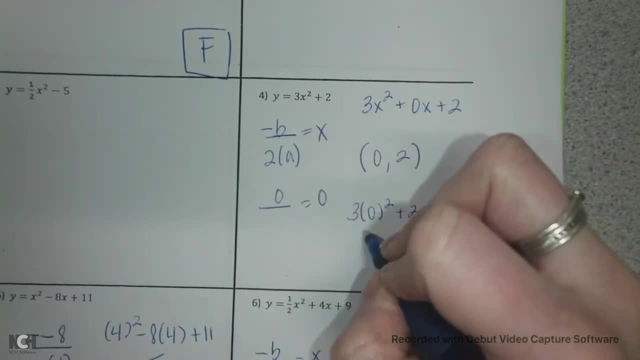 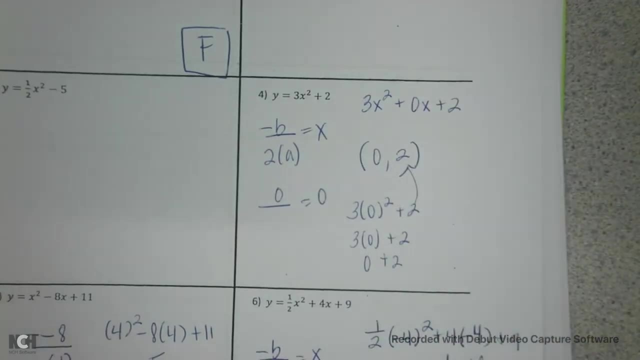 have 3, 0 squared plus 2, it's going to be 0.. So I'm going to plug that in And then I'm going to do: 0 squared is 0.. 3 times 0 is 0.. Plus 2 is just my 2.. So my vertex is at 0, 2.. And it opens up. 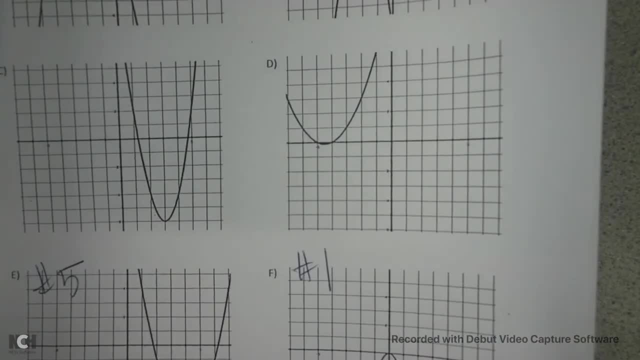 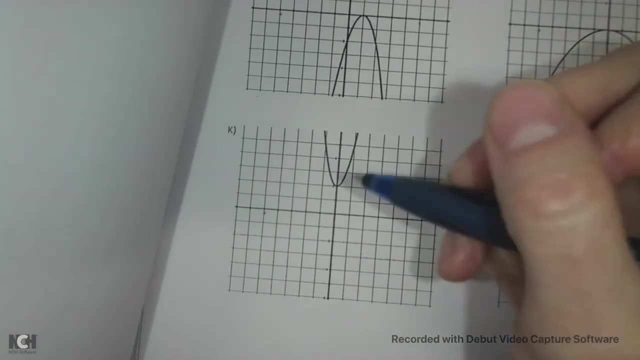 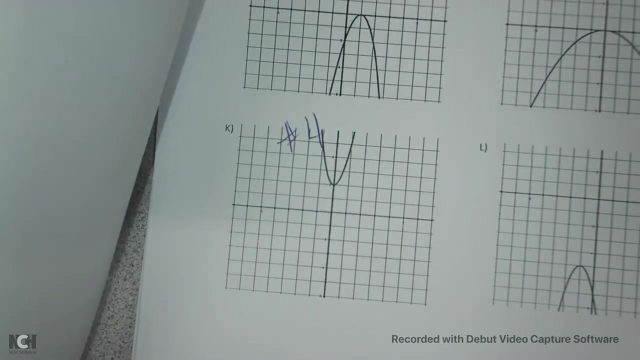 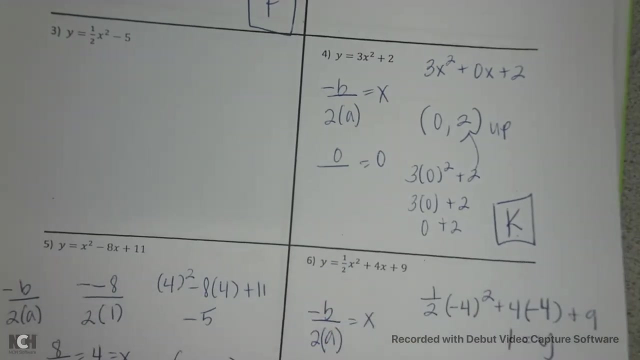 at 0, 2.. So then I will go over here: 0, 2.. Okay, 0, 2.. And it opens up. So which number was that? 4.? Number 4 is k. All right, Keeping that idea in mind, there was one that I wanted to show you. Hold on. 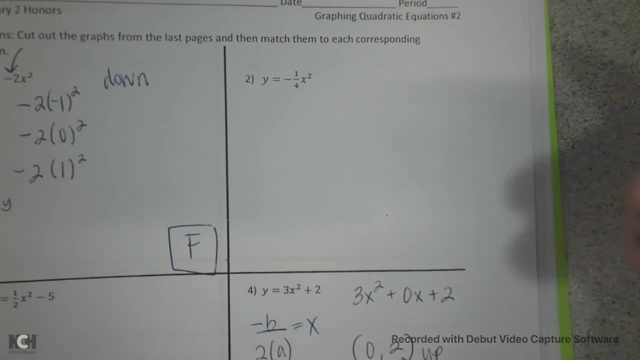 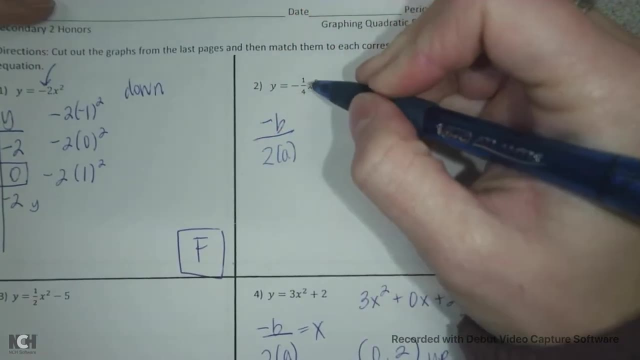 So I wanted to show you number 2.. Let's say I use that same idea If I did negative b over 2a. well, if I'm looking here, I don't have a b value. So not having a b value that's going to give me. 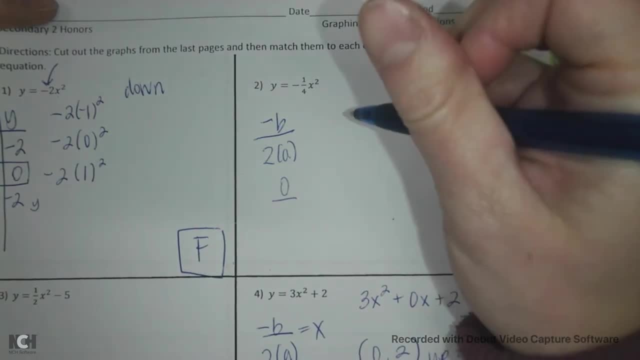 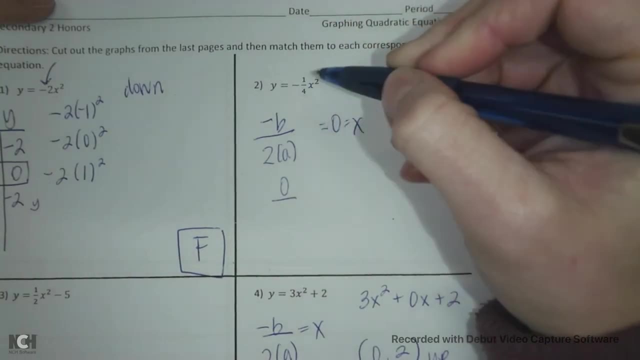 a, 0 for my b, And then, honestly, it doesn't matter, My x value is going to be b or 0.. Okay, Then I plug this guy in. Well, this is negative 1 fourth times 0 squared, So that also will be 0.. So my vertex is: 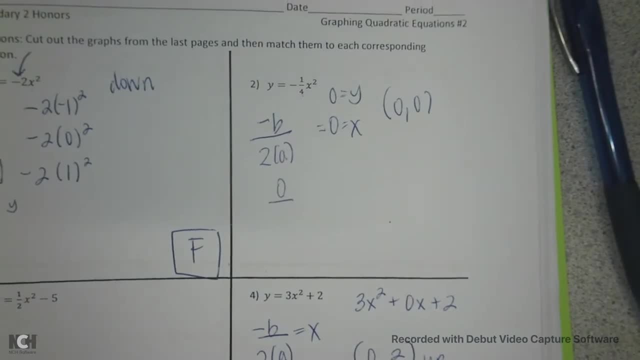 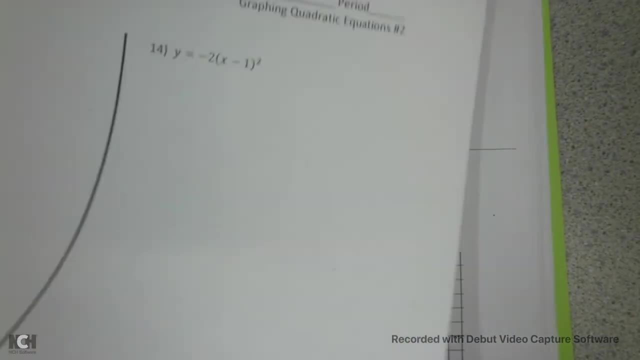 going to be on 0, 0.. Now here's the problem. Also, it opens down because there's q little negative. So we do know that. But the problem is that I have more than one vertex at 0, 0 opening. 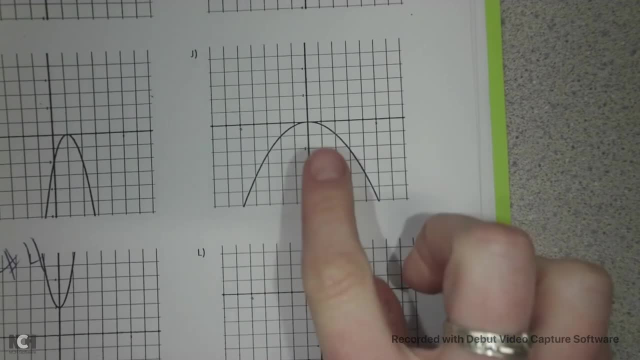 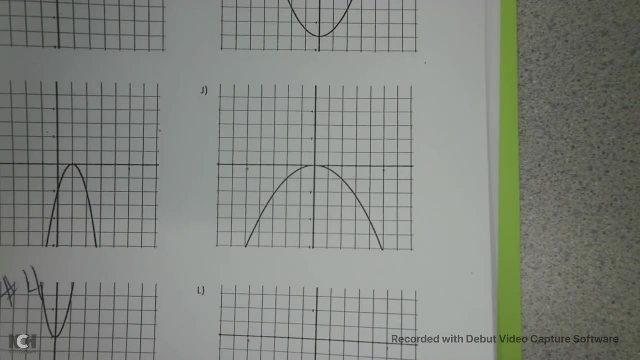 down. So I have this guy, which we already figured out, And then I have this guy, Okay, And then I think that's it Okay, Just those two. So since I already figured out the other one, then I know that it's. 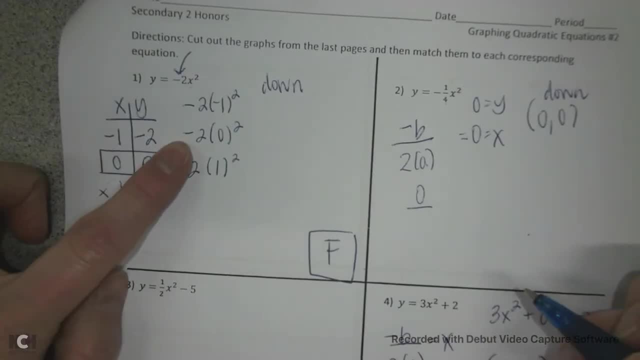 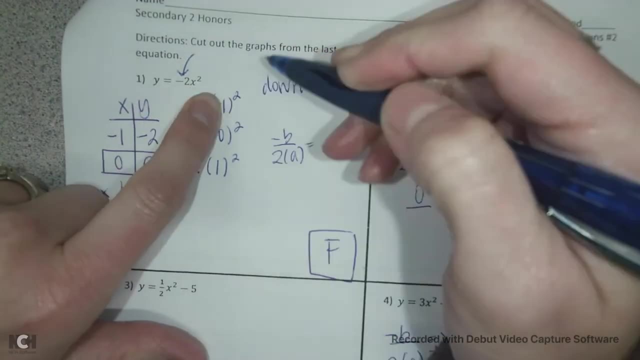 j. But here's the thing: If I would have done negative b over 2a with 1, I would have gotten that same answer. So negative b over 2a. my b value again is 0. So that means that my x value 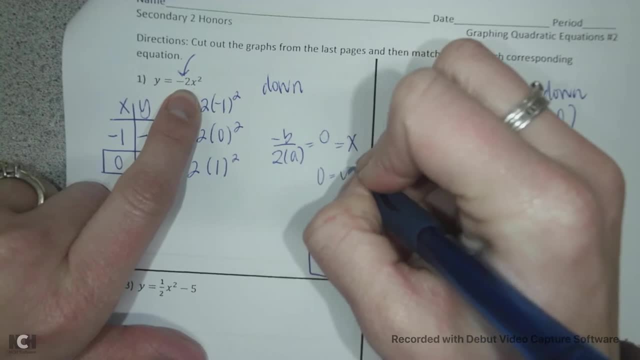 is 0. And then when I plug this in, I would get my y value of 0. So my vertex is going to be 0. So that means that my vertex is at 0, 0. So see how they have the same vertex. So if you do negative, 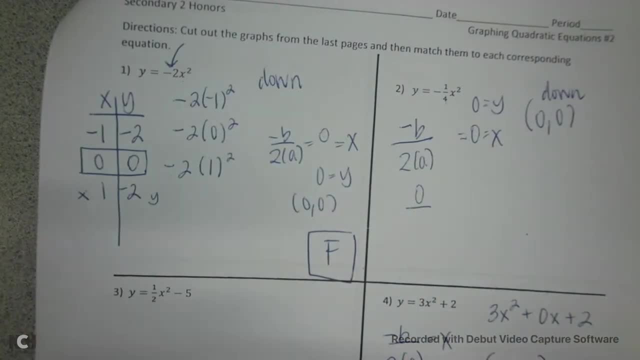 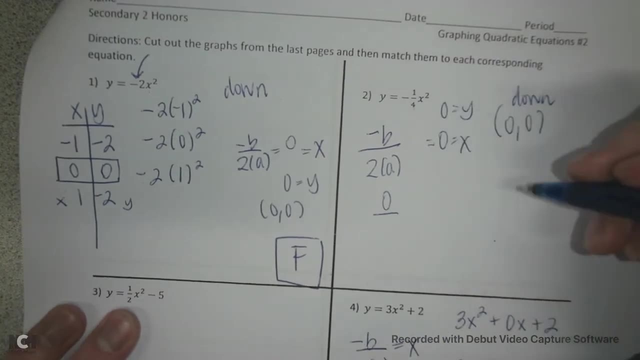 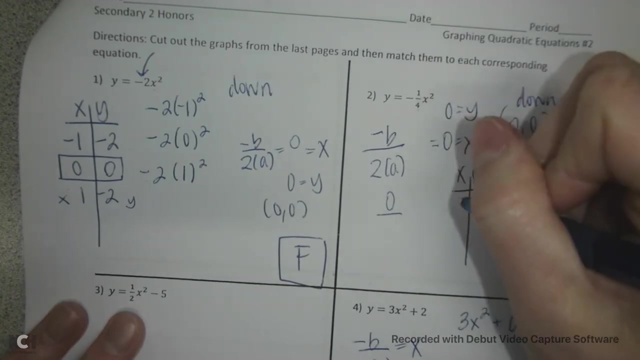 b over 2a, that's totally fine, But then after you might have to make a table of values in order to figure out which graph is which. So, like here, I would just pick a number to make for my table of values so I could calculate. if this is it So, I maybe would pick 1, because 1 is nice, So negative. 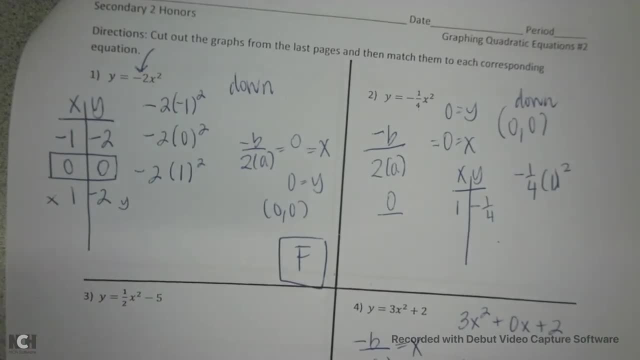 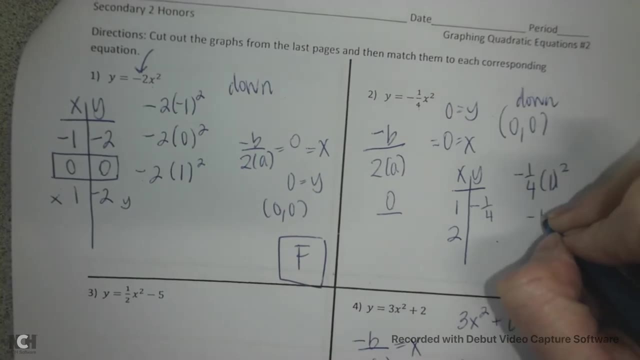 And that gives me negative one-fourth. Maybe that's not the best number to pick, So we would need something. Oh, two, Two would be good. So negative one-fourth times two squared, Because I know if I get a four in here, I know that four divided by four is going to be pretty. 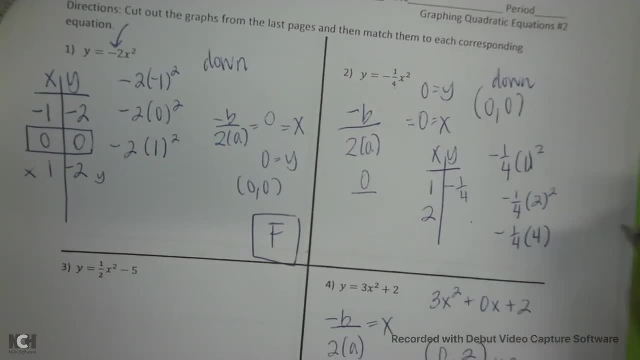 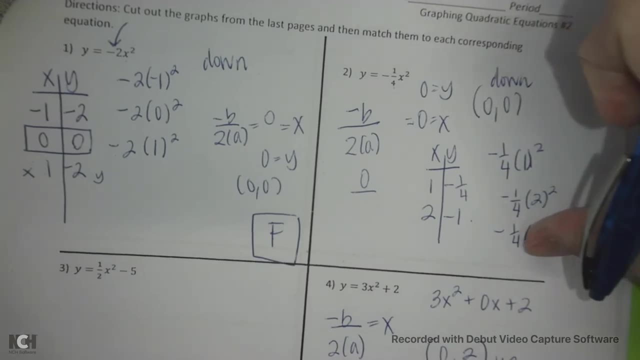 So two squared is four. Negative one-fourth times four is going to be negative one. So this guy should have an intersection of two negative one And, honestly, one negative one-fourth. But that kind of stinks. So two negative one. 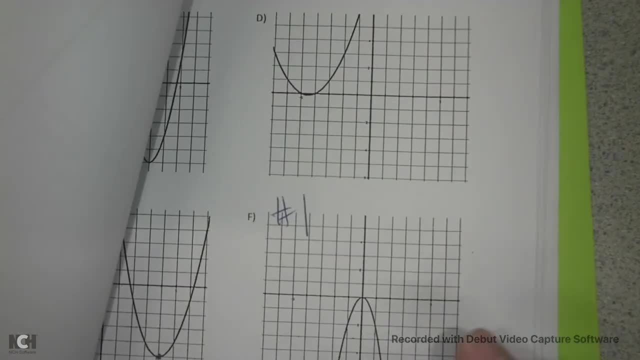 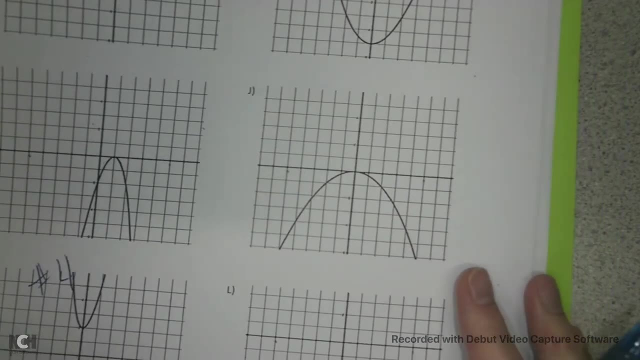 So look for zero-zero and two negative one. So here is the zero-zero. Two negative one is not there. Okay, So it's definitely not F. All right, So zero-zero, And we said it was one and a fourth. So yeah, it actually is looking right. 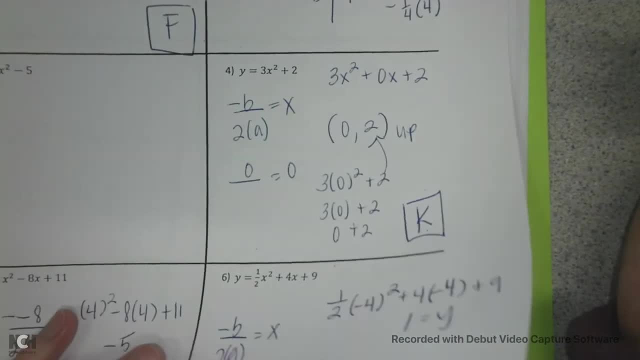 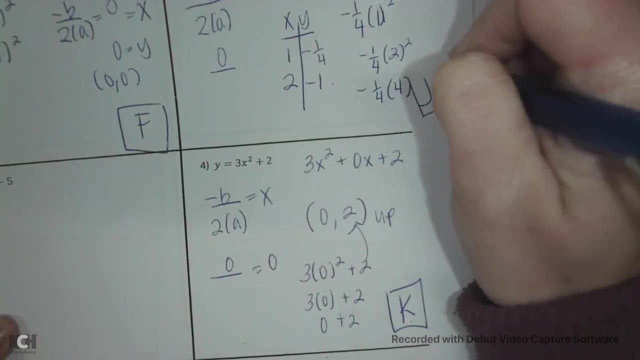 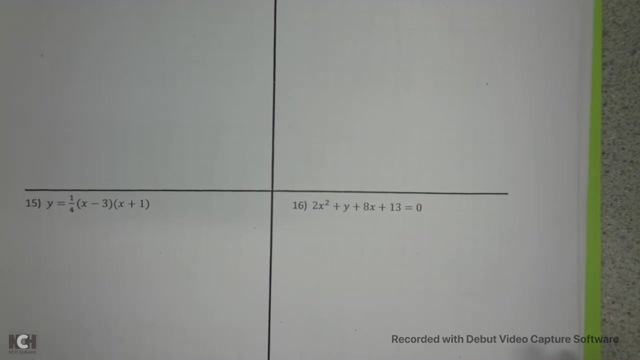 And then two negative one. So for sure, J matches with number two, Okay And J All right. So there you go. There is all of the things, Okay. So remember you might have to manipulate this. so this is in a better form. 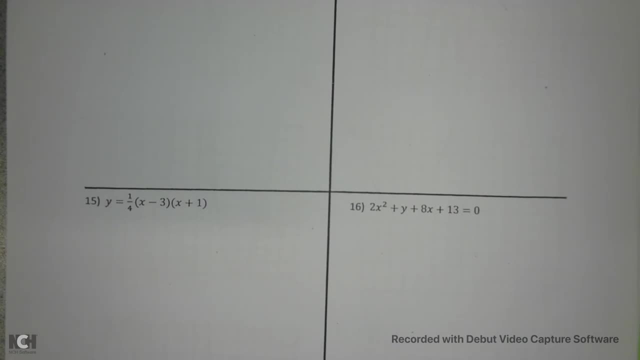 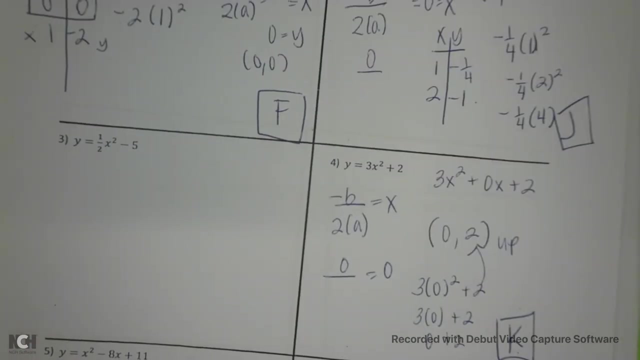 This, you might end up like wanting to multiply through. You have the options to pick what you would like to do in order to figure out which of these match. So good luck and have lots of fun. Bye guys.